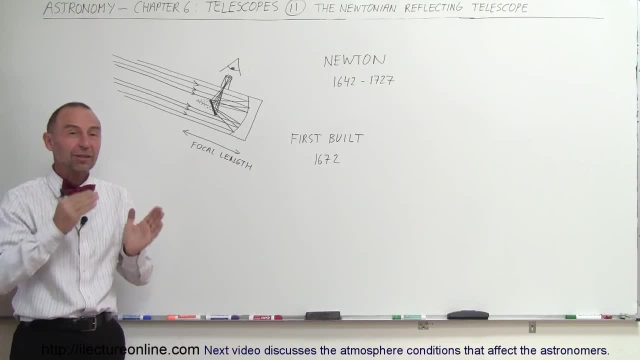 the larger the objective lens had to be. And since it was made out of a solid piece of glass, the weight would begin to deform that glass and made it difficult to keep a good shape and keep a good image, a good, sharp image. with these refracting telescopes, Already many hundreds. 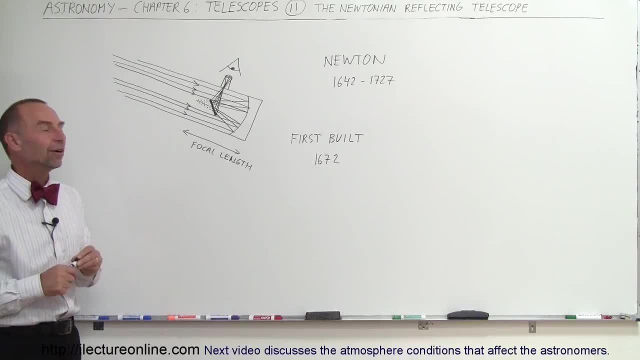 years ago, Newton came up with a very ingenious device in building a new type of telescope called the Reflecting Telescope. So instead of having the light come through an objective lens and refract or bend the light, Newton built a telescope with a mirror at the very bottom of the telescope. So 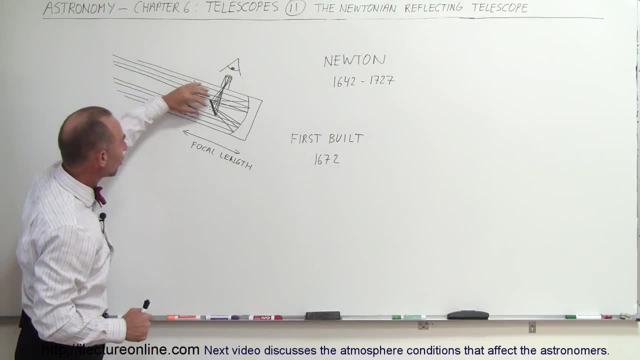 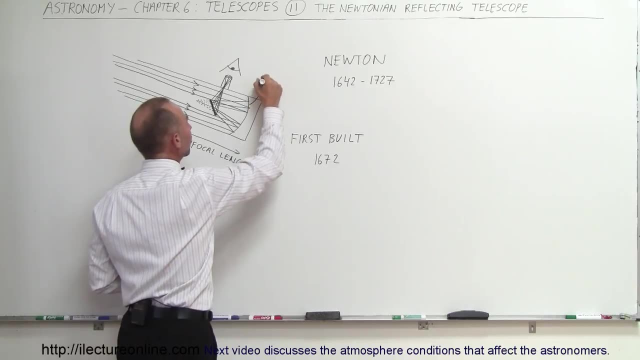 at the top. the telescope was open. The light could come in through the open part of the telescope and bounce off of the telescope. So it was a very ingenious device And it was a very ingenious place in which a light would come out, bounce off the person and then it would bounce off the 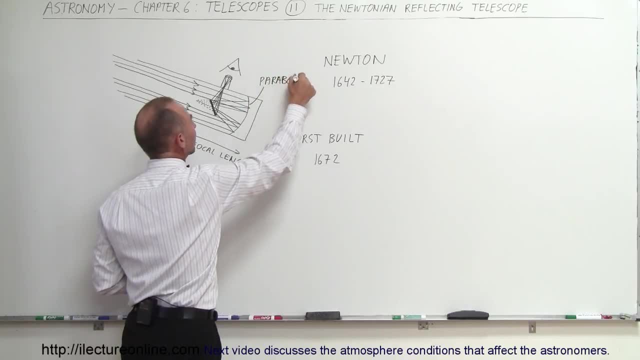 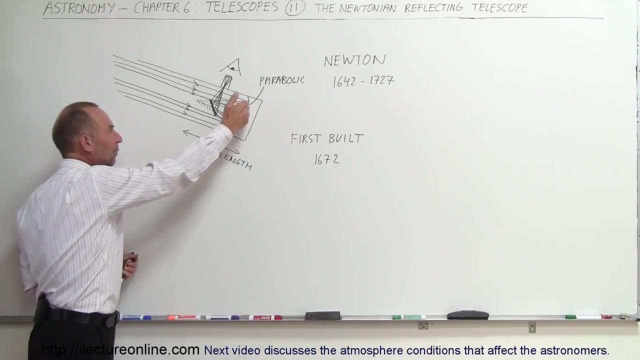 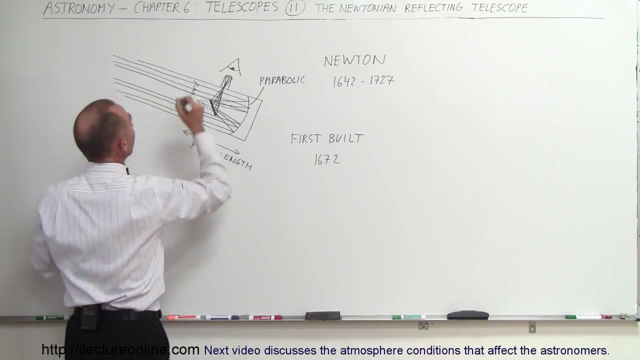 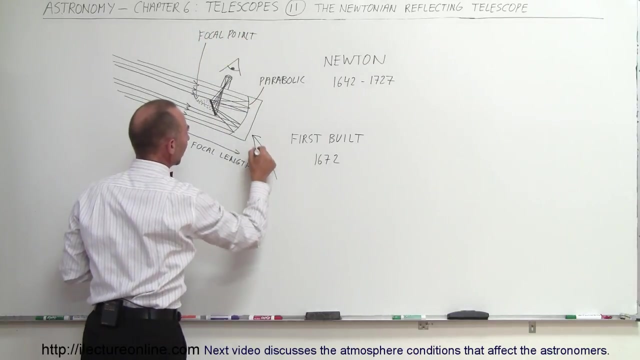 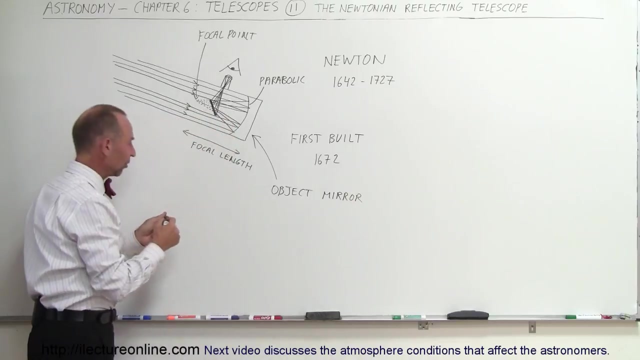 Cambodia: The導 the Mirrors. Мейг الdate О NPC 箱. to see how the objective mirror in this case- So objective mirror, it's not a lens- and so the light would then be reflected back, but before it came together here at the focal point, you would put a mirror in its place, a small mirror at an angle. 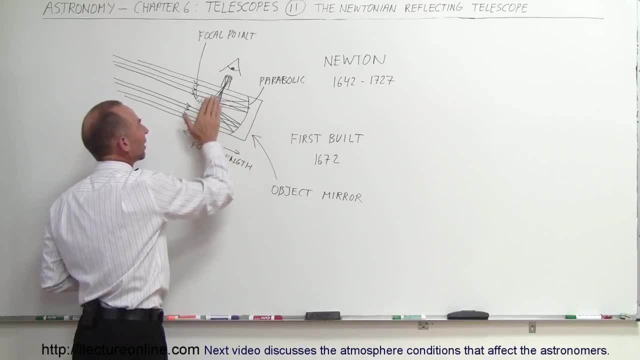 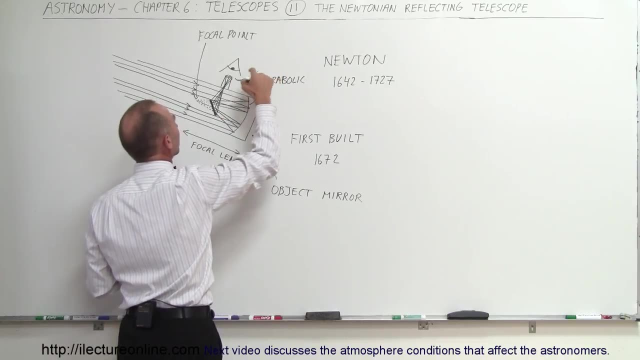 so the light rays that are reflected would bounce off the mirror, reflect in this direction and then finally, with a small eye piece over there, you would then look at the telescope in that direction. So, and I should go this way, this is called the eye piece through which you would see the image, and the image would then form. 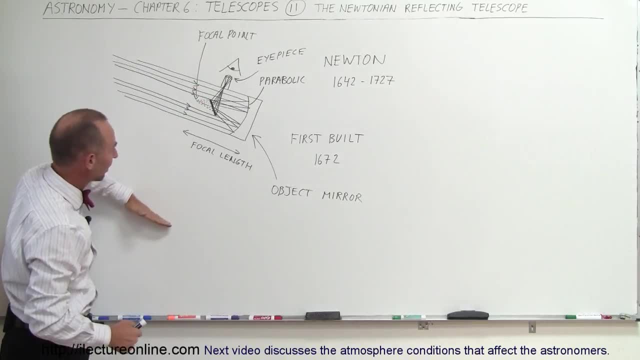 it would then, of course, be a virtual image that would form somewhere out here in the direction that they're looking. it would also be inverted or upside down, and it would be a virtual image indeed. But what is the big advantage to having a telescope like this versus a refracting telescope? 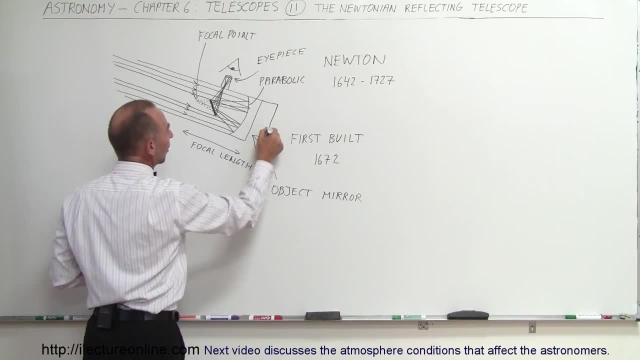 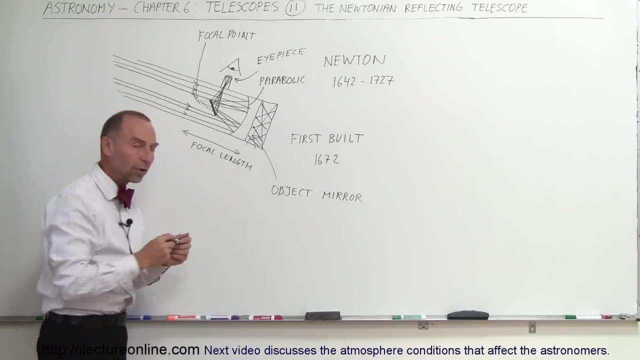 Well, for one, you can make these lenses very big. You could put a very big steel supporting structure at the bottom of the telescope, right there, and to hold the mirror in place, regardless how heavy it was, you could build a very strong structure so that the mirror would stay perfectly shaped the way it was meant to be. 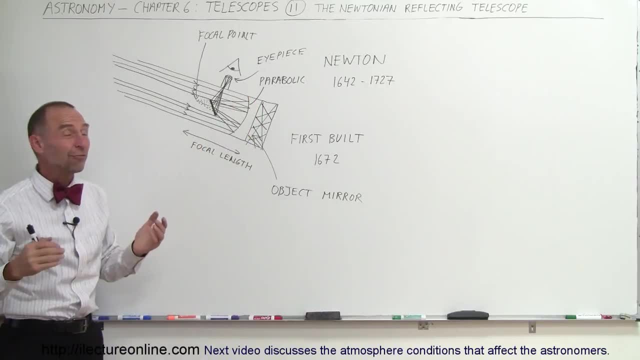 and it turns out that using this technology we've built some very, very large telescopes. The largest one that we built here in the United States was five meters across the Hale telescope and the mirror weighed thousands of pounds, probably several tons of mirror that we had to build here at the bottom. 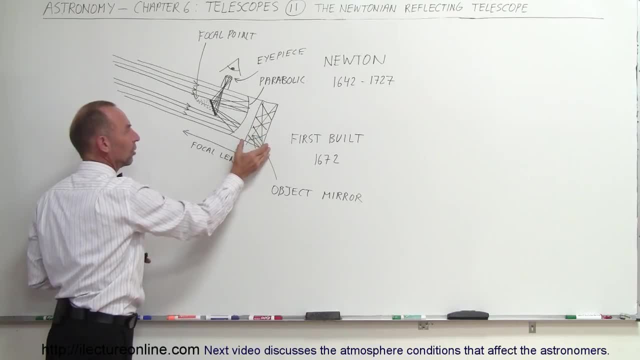 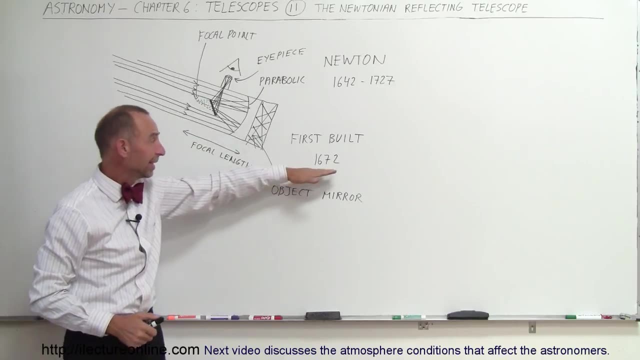 and nevertheless it was a very, very big telescope. And it was a very, very big telescope. It has that very strong steel structure not getting in the way the light rays would then be able to support that mirror. So this new design that was built, this mirror was built in, or this telescope was built in 1672 by Newton. 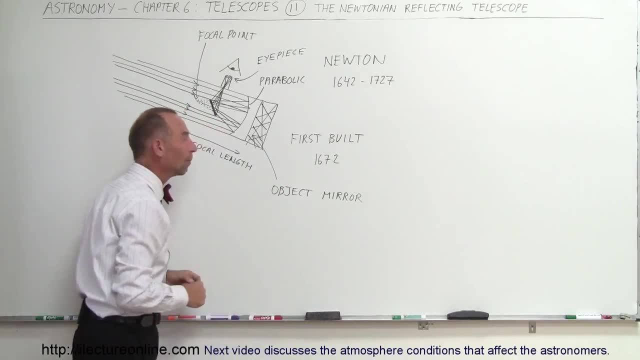 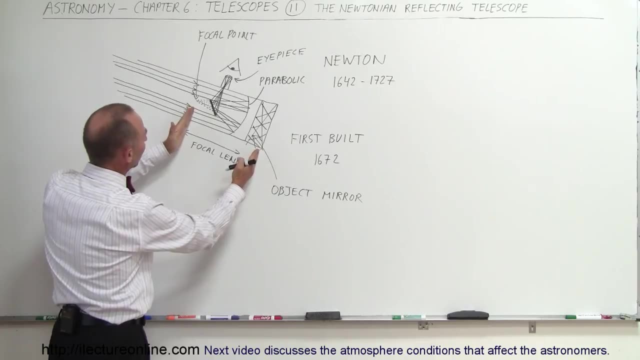 notice, Newton was about 30 years old when he built that telescope- Very ingenious to come up with this design. Now, what happens, though, is that the focal length of these telescopes tend to be somewhat smaller. these tend to be shorter. of course, some of the very big telescopes have now been adapted to this. 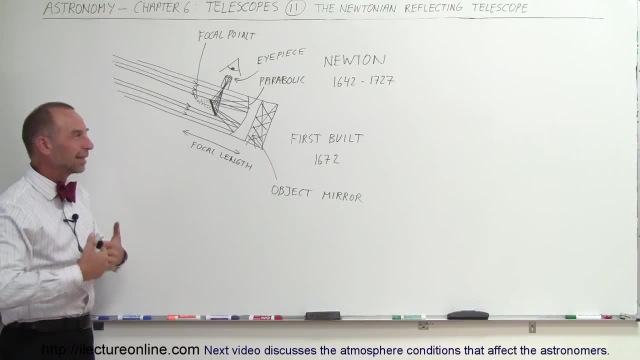 have very long focal lengths, because the longer the focal length, the greater the magnification. and yes, with the very big telescopes we wanted the big magnification. Some of you may say, well, wait a minute, this mirror here that gets in the way, that would then block out the light coming in this direction. that's indeed the case, so you wouldn't get. 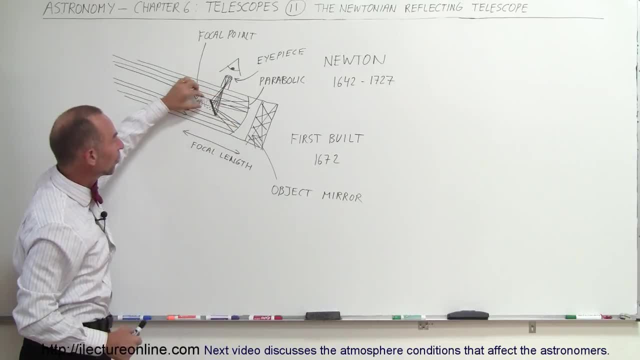 the advantage of having the collection area of the entire mirror, but a small portion of it at the center of the mirror would be blocked out by this mirror here. that would then reflect the light into the eyepiece, and then you may also say: well, doesn't that get in the? 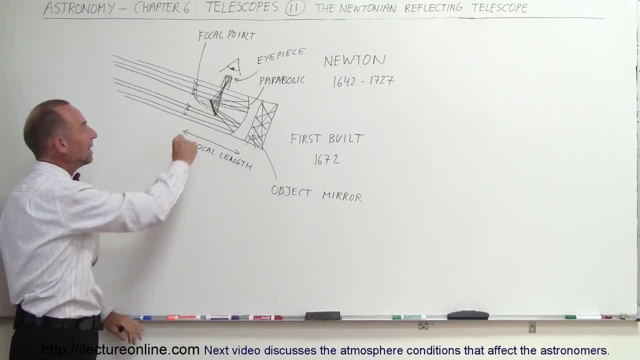 way. doesn't that kind of block part of the image? and the answer is no, Any portion of the mirror here. and of course, remember, if you look at the mirror, the mirror would look like this and then the central portion would simply block out like that. so 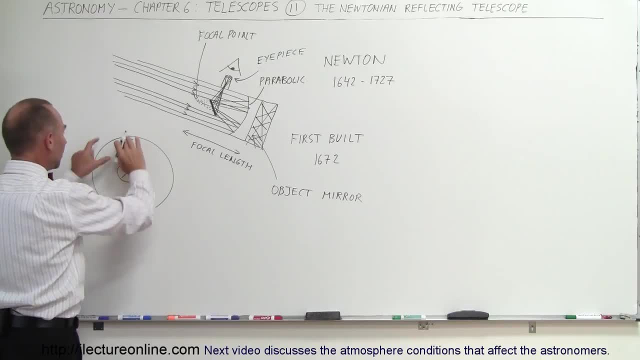 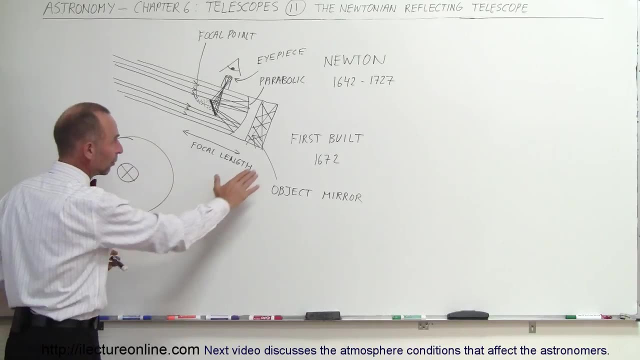 this would be blocked out by the reflecting mirror right there. but this rest portion, the other portion of the reflecting mirror, or I should say the reflecting objective mirror, there This would still be a large percentage of the total area of the mirror. so you don't lose much of the image, you don't lose much of the photons that you'd be able to collect. 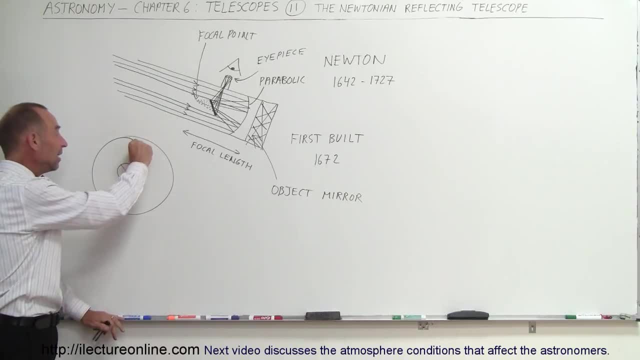 and on top of that, this would not get in the way at all. you would not see it, because any small portion of the mirror could generate the entire image. so therefore, when you put something in the way, you don't see it at all. What's even interesting is, if you take a look at, if you take one of these telescopes, you